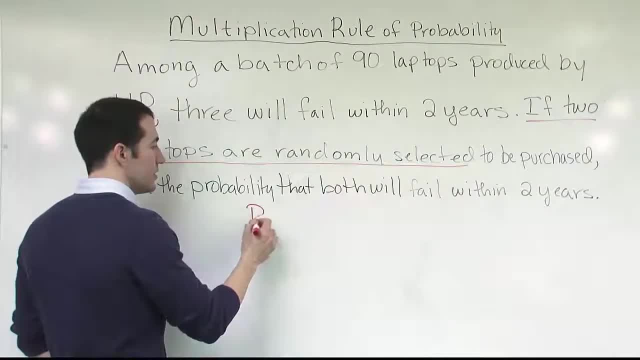 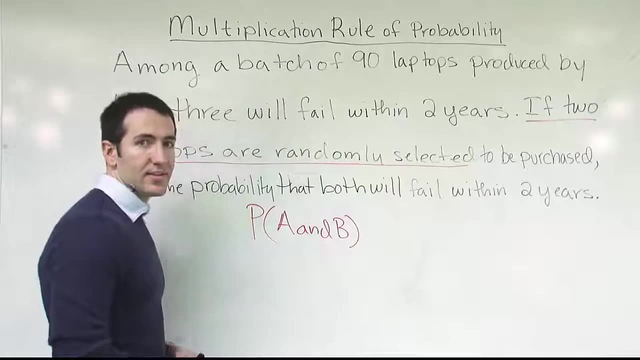 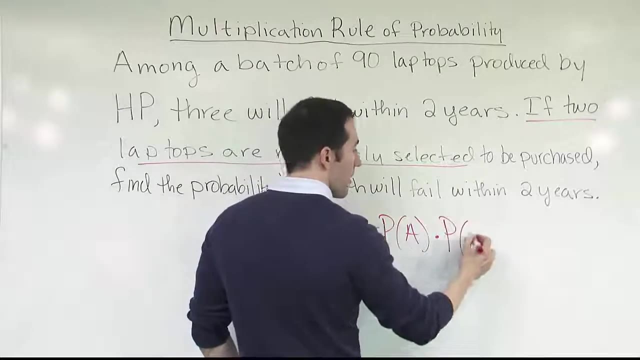 Before we start the problem, I want to look at the formula just in the abstract sense. So the probability of A and B for the dependent case works out like this: It's going to be the probability that A occurs times the probability that B occurs. 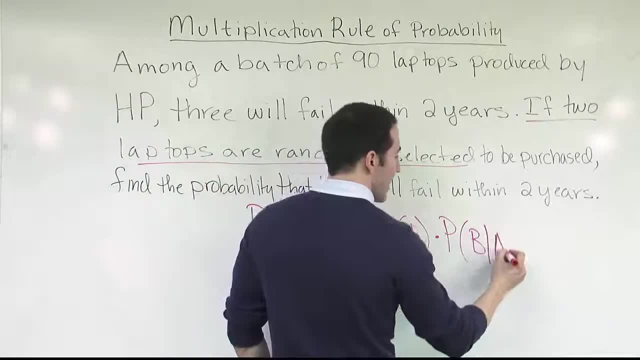 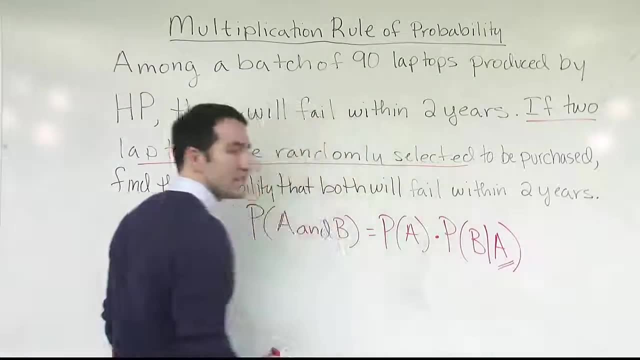 That seems natural, but we're going to add a little extra thing here, Given that A has happened or has occurred. So this part is very vital. What this means is that when I go to work out the probability, the first probability I calculate right. 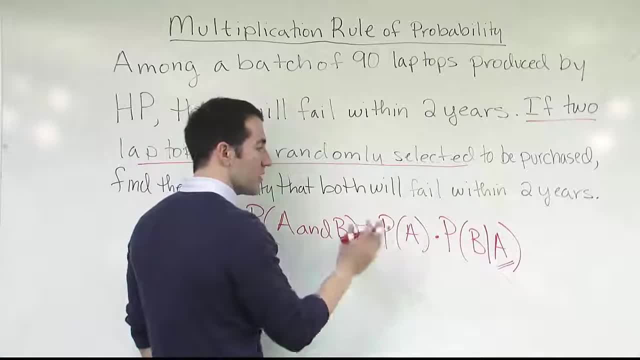 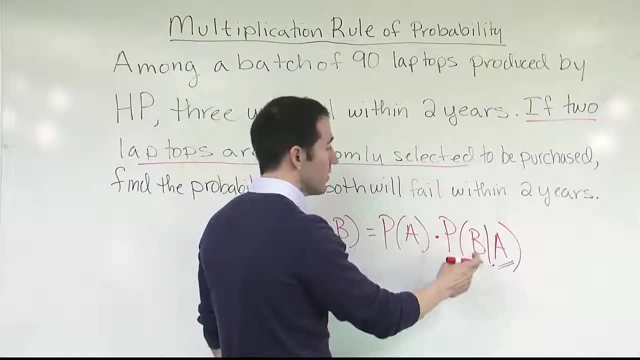 That's just going to be the probability that A occurs. That's just a basic probability. that's pretty straightforward. Nothing new there. When I come here, though, when I go to work out the probability that the second event occurs, the event B occurs. 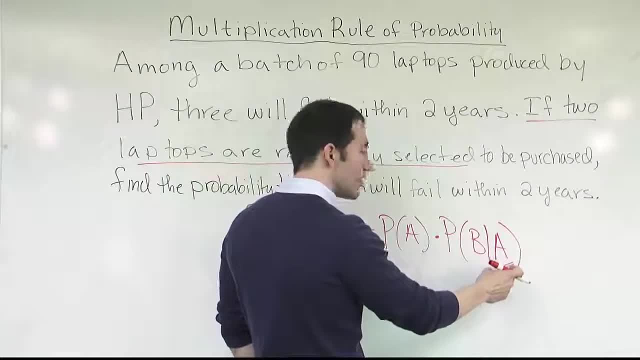 I have to pretend that A has happened, I have to imagine that it occurred like it was supposed to. So I'm not thinking: well, maybe it didn't occur, or maybe it did occur. I'm going to say no, no, it did occur. 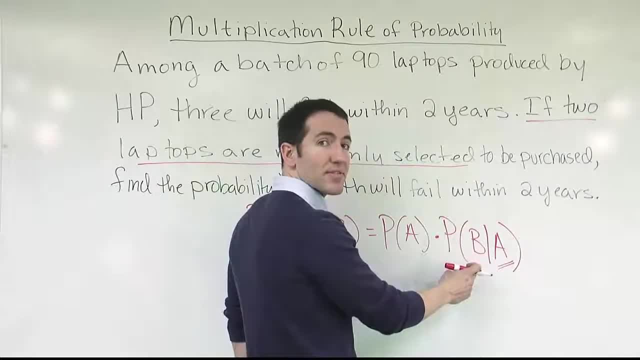 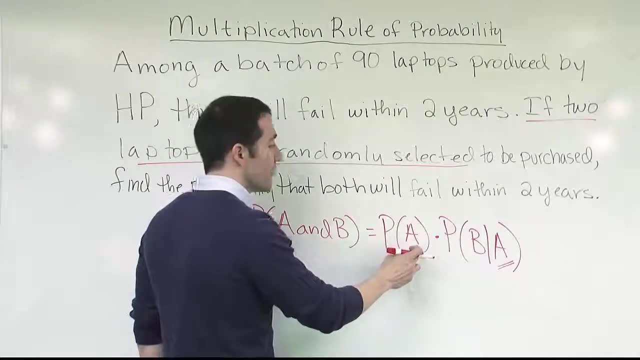 It happened And because it happened, how does that affect B? That's what I have to take into consideration. So remember, when we do this problem, we're going to assume that the first thing turned out the way we said. We say probability, that the thing is red. 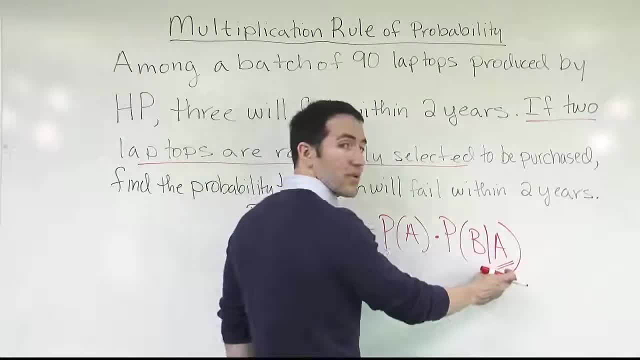 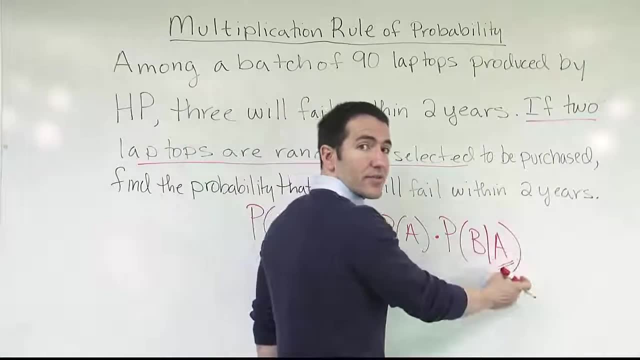 Then we're going to consider over here probability that B occurs, given that the thing was red, right. Whatever, If I say probability that the first one is defective, then the next one will be probability that B occurs, given that the first one was defective. 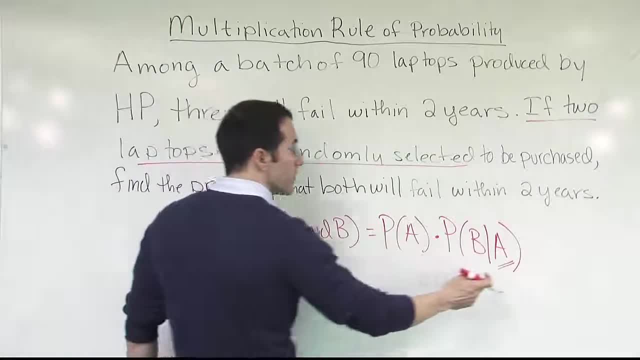 That has to be the way it's done. So that's very important, Because otherwise you start getting into this mind game where you say, well, what if it didn't turn out the way it was supposed to in the first step? Then things would be different. 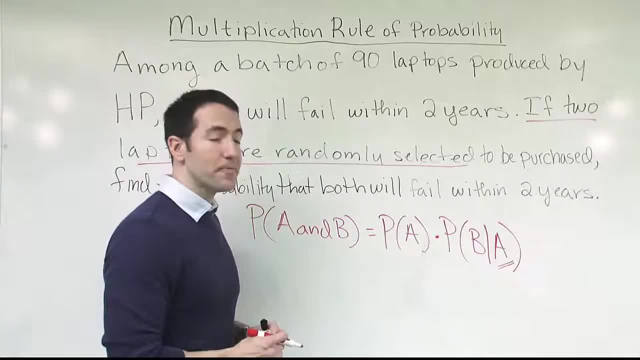 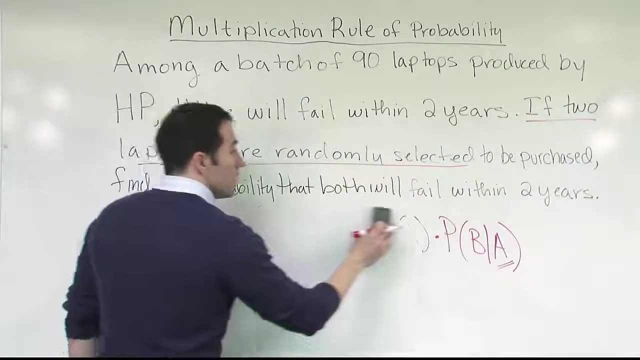 And then you're going to get into a much more complicated way to calculate the probability. So let's go ahead now and actually work out this particular problem. So what we'll do is we'll start out by writing the phrase if two laptops are randomly selected to be purchased. 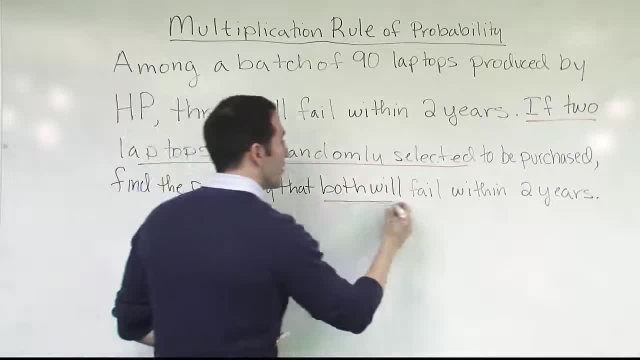 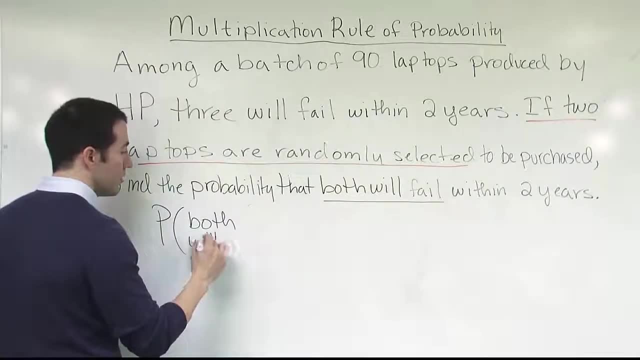 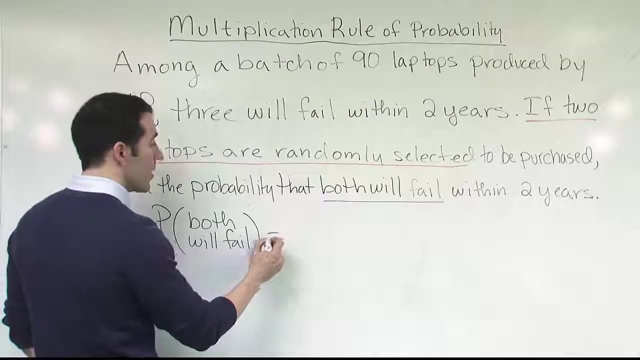 find the probability that both will fail. Both will fail. So I'm going to write that as a probability right, Probability that both will fail. Okay, So that's my probability statement, directly taken from the problem. Then I'm going to say okay. 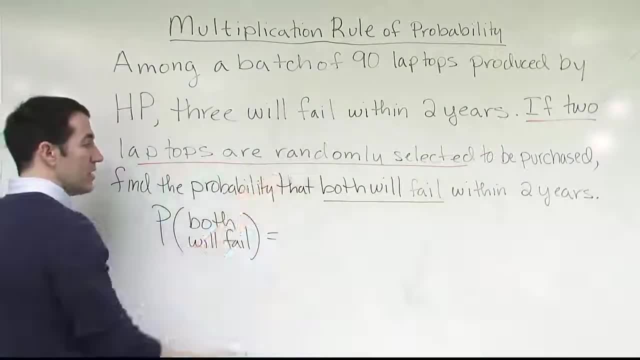 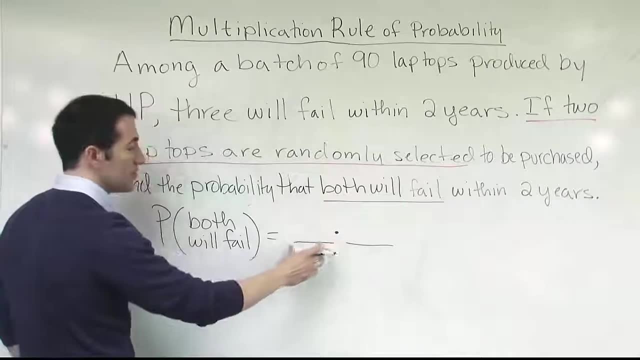 the fact that I'm selecting two laptops at random means, I'm going to have remember two spaces to place probabilities. That two is to be used here, right? It's used to tell me that I have one probability multiplied by another probability. 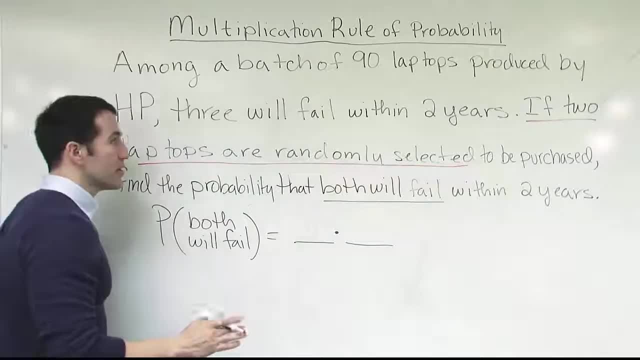 Once I've used that two, it's all used up, It's spent, I won't use it again. So I basically kind of cross that off and think I'm not going to put a two in my fraction somewhere here because of that two. 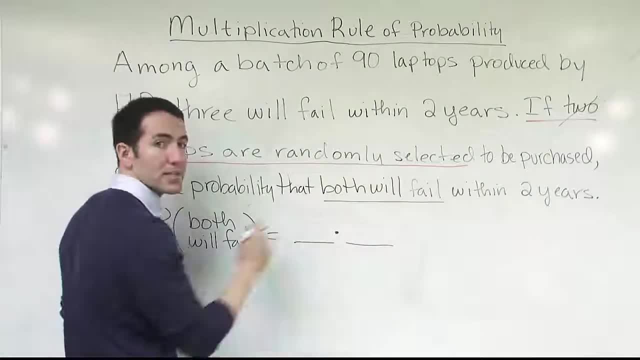 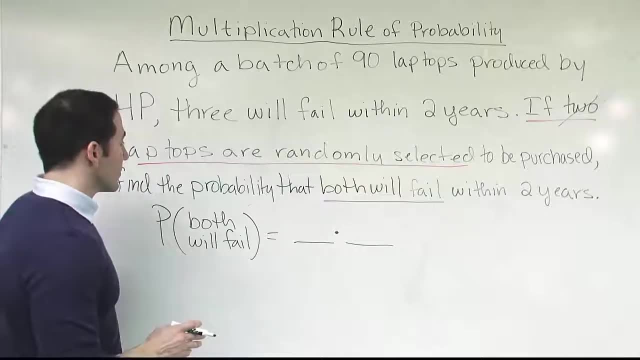 That two is used up. once I realize that it tells me I have two spaces for probability, The other rule was to tell me that it was a multiplication rule. Now it's done, I won't use that information again. All right, Now what I do have to look at then. 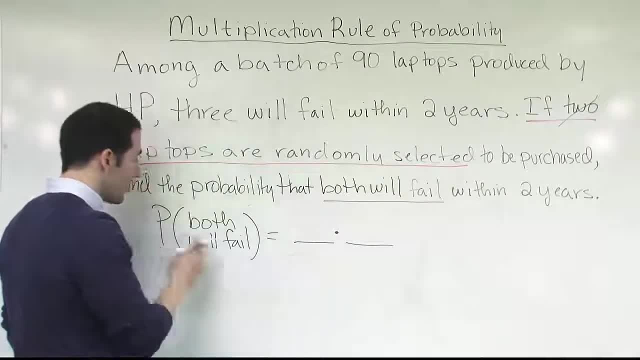 is what does this first fraction represent? I want them both to fail within two years, right? So not that I want that, but that's what the probability we're calculating, right, The probability that both laptops would fail within two years. That means I need this fraction to represent the probability. 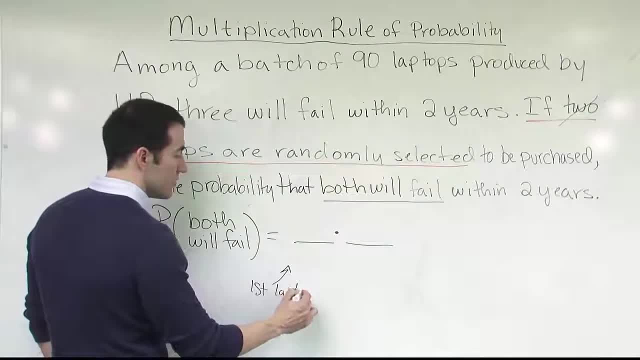 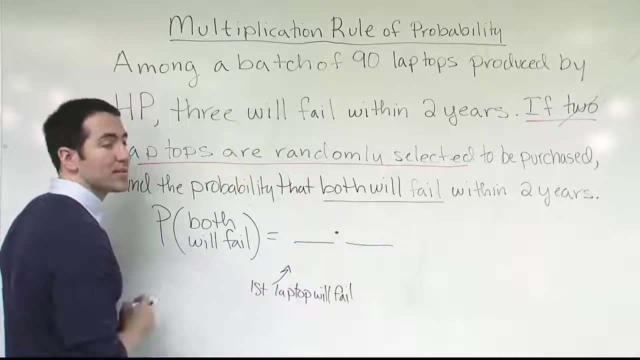 that the first laptop will fail. So, the first laptop I purchase, I want to know the probability that it fails within that time frame. Well, that's basic probability. So I'm going to look at the number of laptops that will fail within two years. 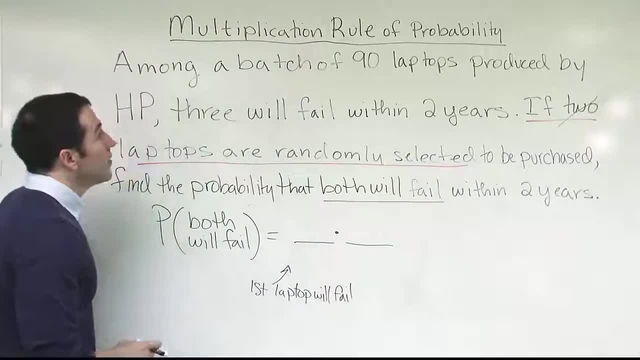 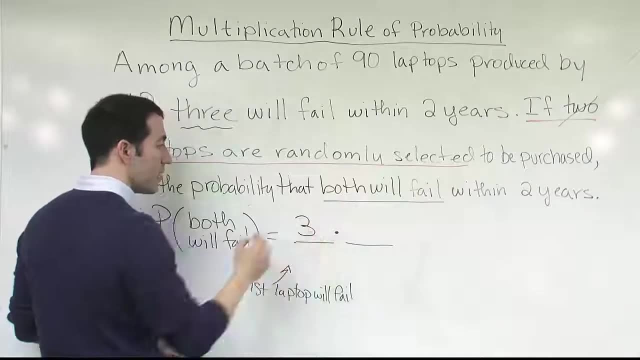 divided by the total number of laptops on the shelf. Well, it says that three. three laptops will fail within two years. So when I first go to the shelf, there'll be three laptops that are defective divided by the total number of laptops. 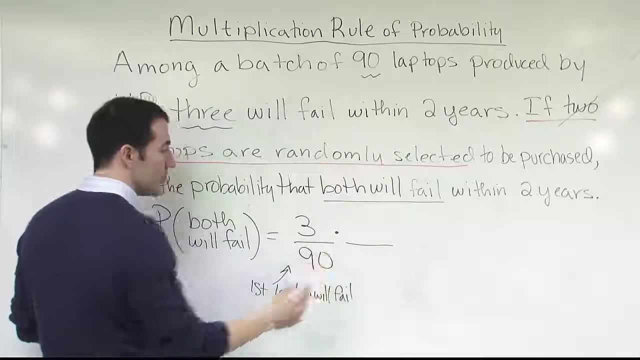 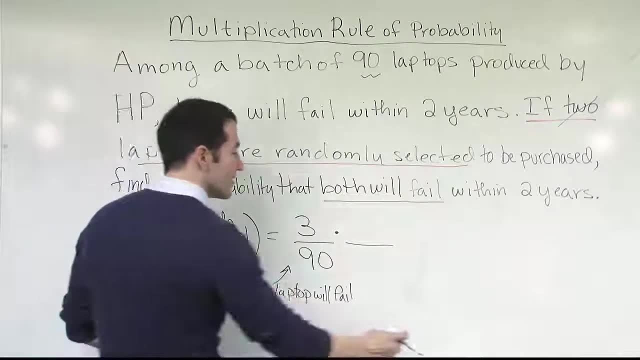 90 laptops, So the initial probability that I'll get of a laptop that will fail is 3 over 90.. That's just your basic probability Now. from there, though, I got to go to the second part of the problem, And here's where things change a little bit. 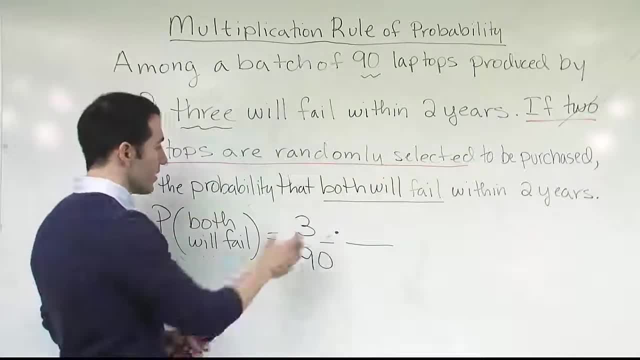 And this is where we have to worry about the dependent scenario, Because we're going to say: hey look, we went to the shelf. the probability that I got a defective laptop was 3 over 90 when I went to the shelf the first time. 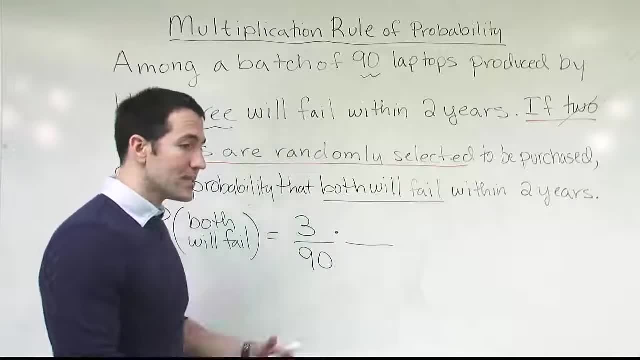 I picked that laptop up, I put it in my cart right, I go back to the shelf and I realize now the total number of laptops is different. There's only 89 laptops to choose from. That's the first difference. Second thing is: